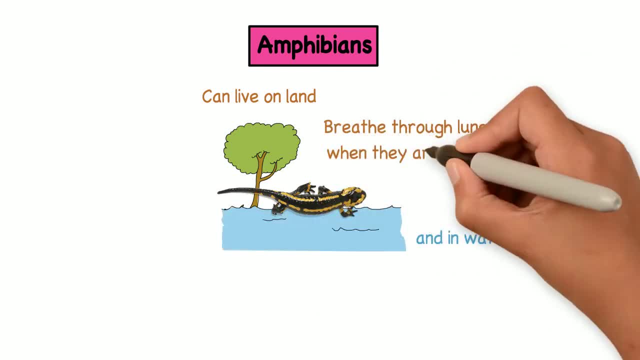 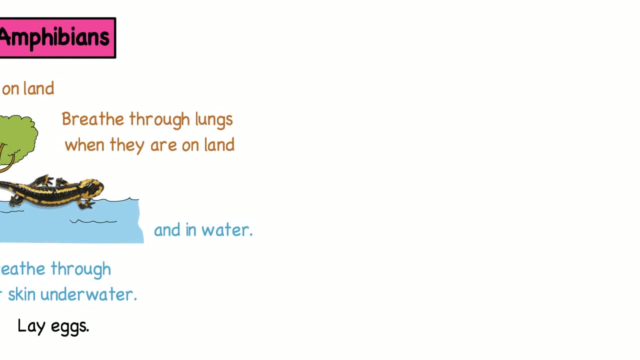 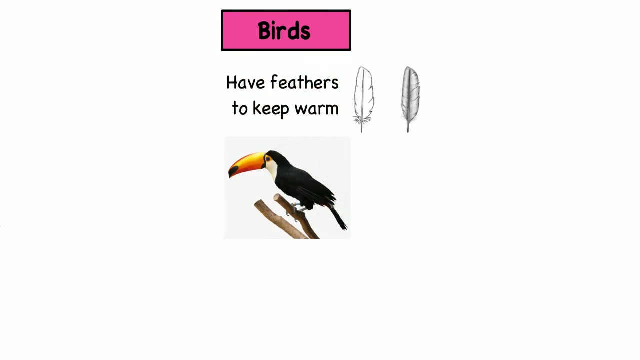 When they live on land, they breathe through their lungs, And when they are underwater, they breathe through their moist skin. They can also lay eggs Birds. They have feathers to keep them warm. They also have a beak and a pair of wings to fly. 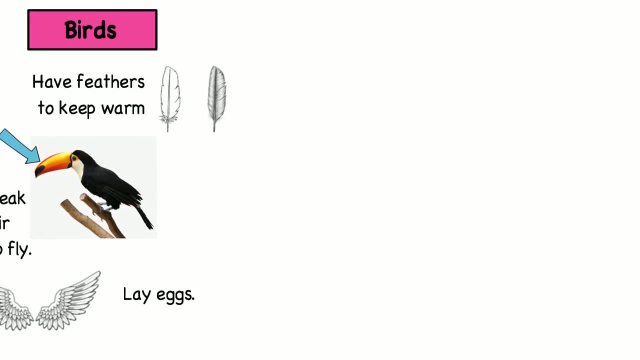 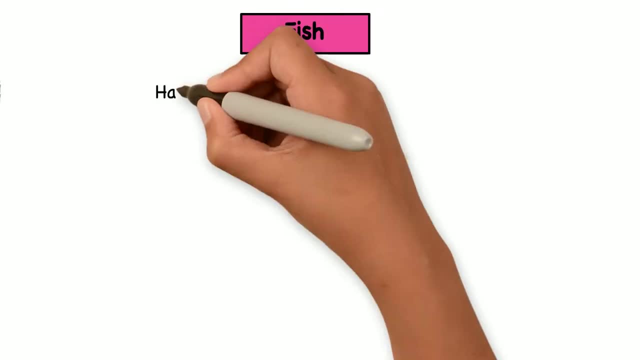 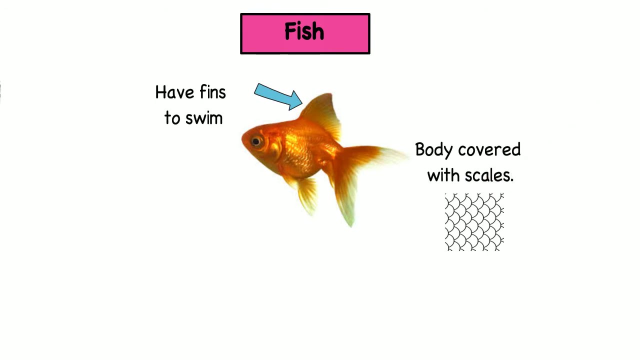 They lay eggs, Fish. They have fins to swim, Their bodies are covered with scales And they breathe through gills underwater. Most of them lay eggs to reproduce Insects. They have three pairs of legs. Can you see them? Insects? They have three pairs of legs. 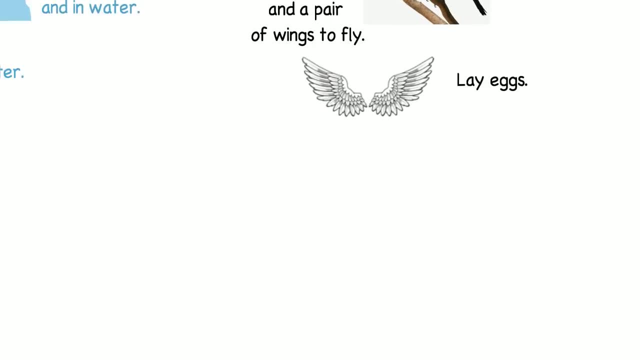 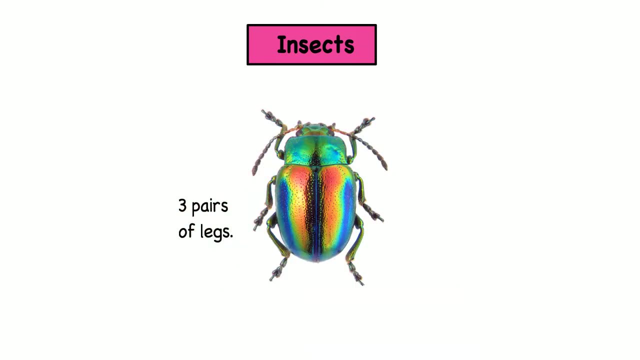 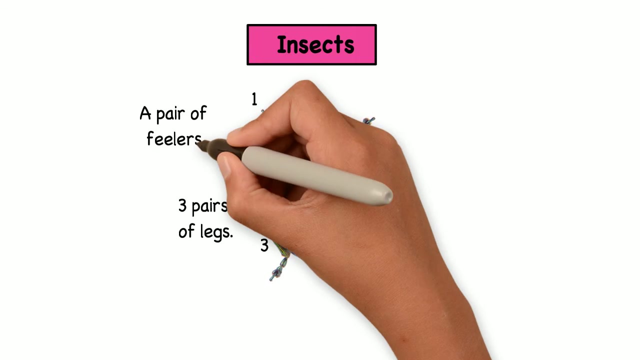 Can you see them, Insects? They have three pairs of legs. Can you see them, Insects? They have three pairs of legs: One, two, three, One, two, three. They have a pair of fillers. They have a pair of fillers. 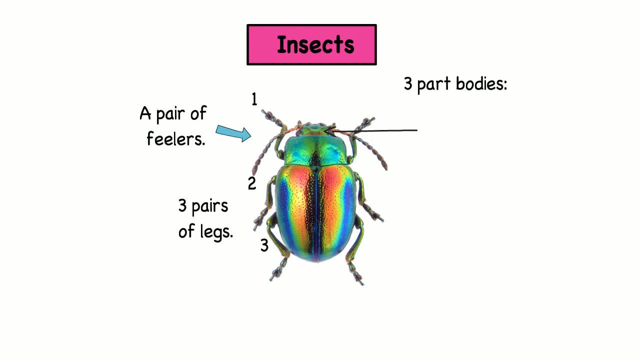 And their bodies are divided into three parts. And their bodies are divided into three parts: The head, The thorax And the abdomen. And the abdomen. And yes, they also lay eggs to reproduce. And yes, they also lay eggs to reproduce. 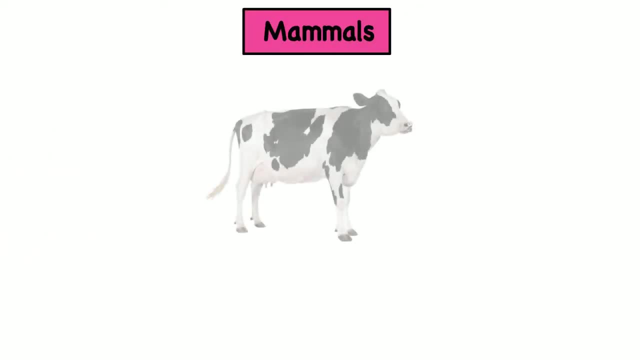 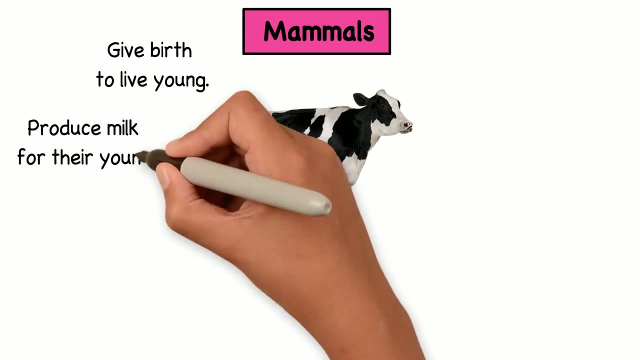 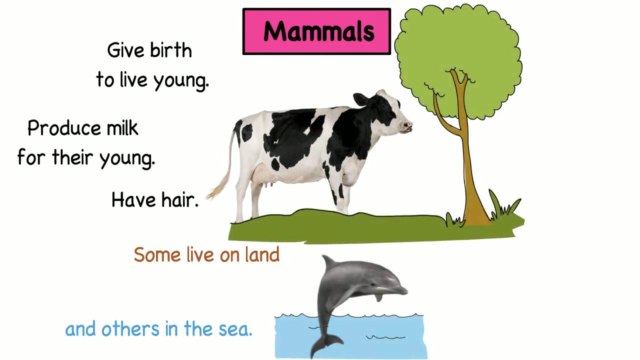 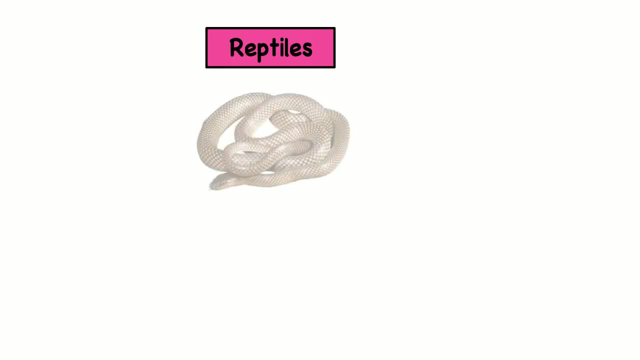 Now the mammals. They give birth to live young, they also produce milk for their young and they have hair. Some mammals live on land and others in the sea, like the dolphin, And now the last group, the reptiles, Which are their characteristics. 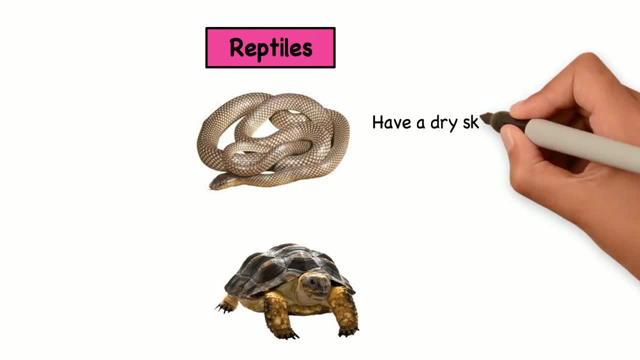 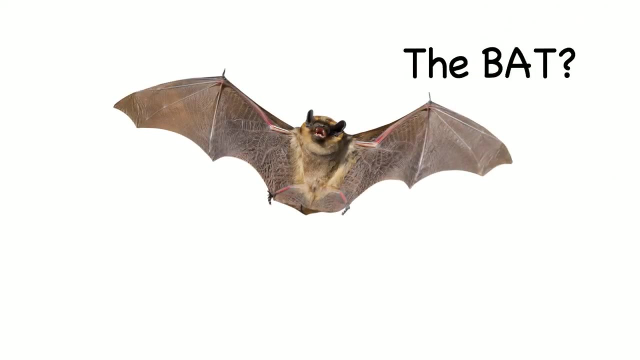 Well, as you can see, they have a dry skin covered with scales and some, like the turtle, have shells. Now it's your turn. What do you think Is the bat a bird or a mama? Leave your answer in the comments. 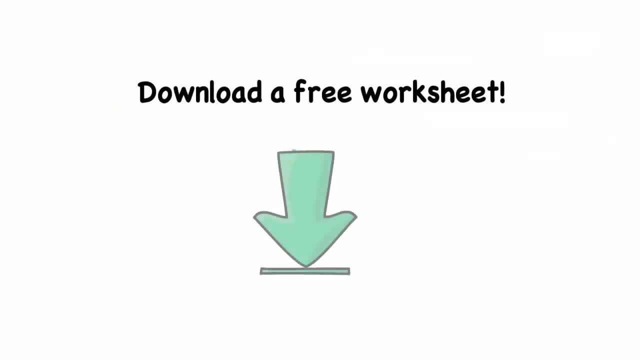 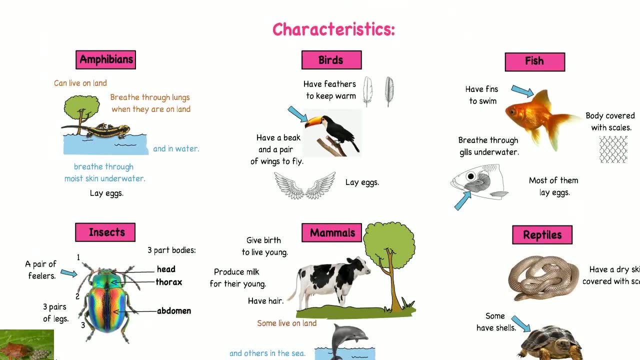 And if you want to test yourself on this topic, you can also download the free worksheet to put into practice everything you have learned about animal classification and their characteristics.